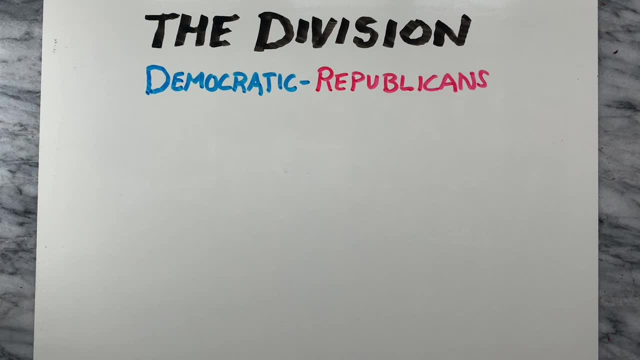 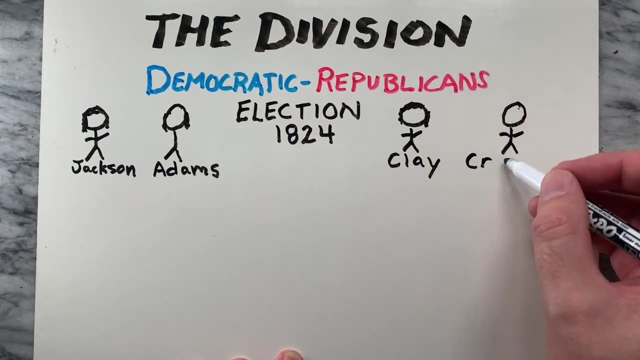 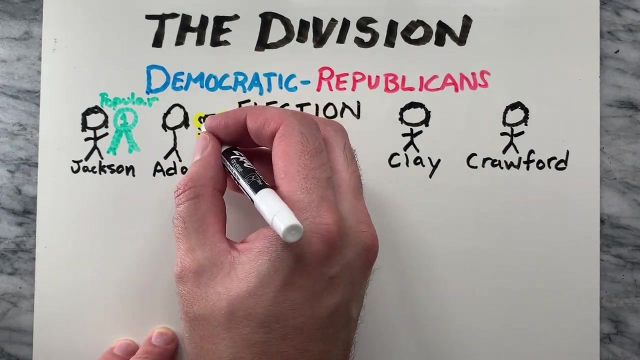 the Democratic-Republicans dominated the political scene, causing the Federalists to slowly dissolve away. Because the Democratic-Republicans were so popular, the party had several political candidates who ran against each other in the presidential election of 1824.. John Quincy won the presidency in spite of Andrew Jackson winning the popular vote. This began a divide. 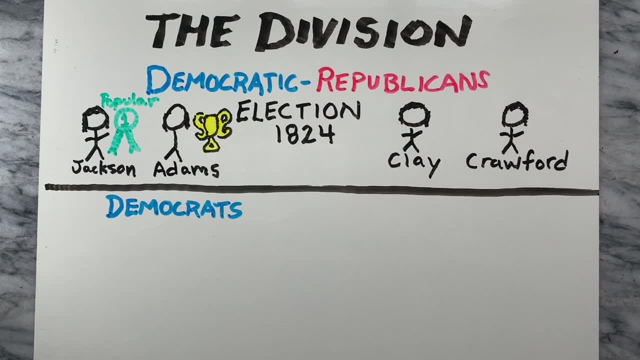 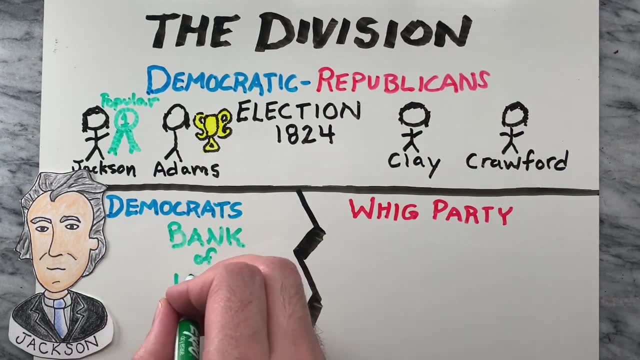 within the party, which eventually caused the party to split in two: The Democrats, or Democratic Party, and the Whig Party. The Democrats were led by Andrew Jackson. he was against the existence of the Bank of the United States and he largely supported State's rights. 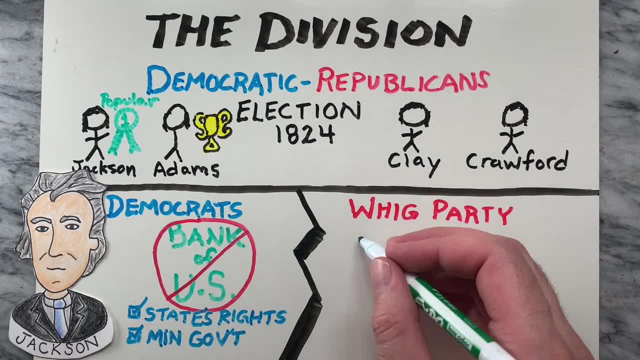 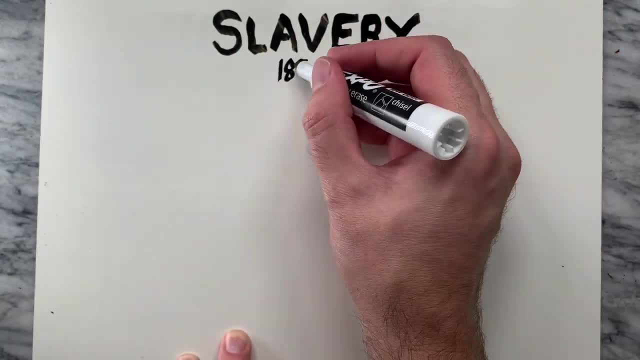 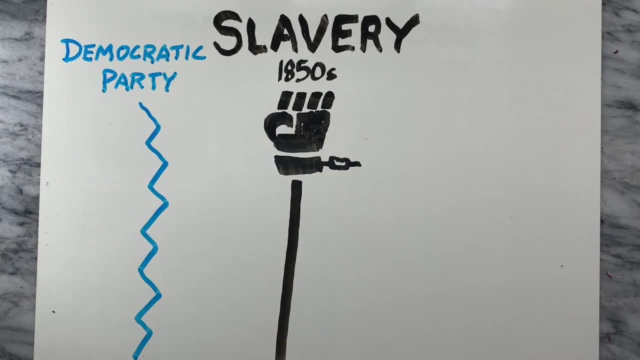 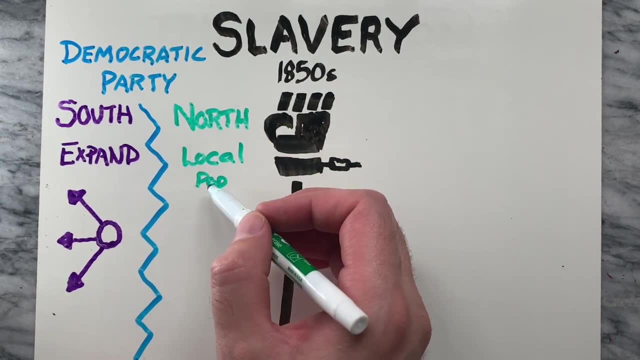 this matter differed greatly. Southern Democrats wished for slavery to be expanded and reach into western parts of the country. Northern Democrats, on the other hand, argued that this issue should be settled on a local level and through popular referendum. The divide in the Democratic Party 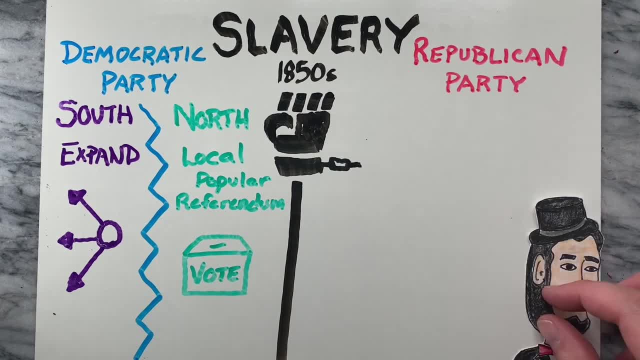 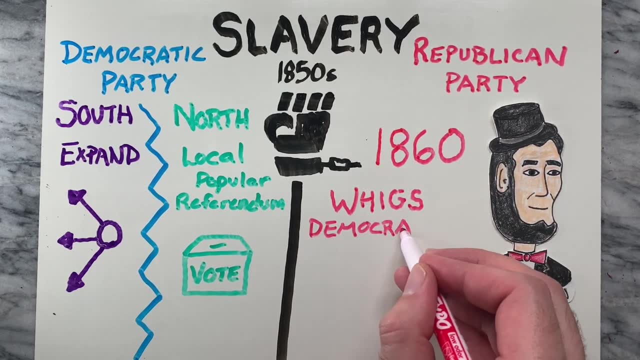 eventually led to Abraham Lincoln, who belonged to the Republican Party, winning the presidential election of 1860. This new Republican Party had recently been formed by a group of Whigs, Democrats and other politicians who had broken free from their respective parties in order to 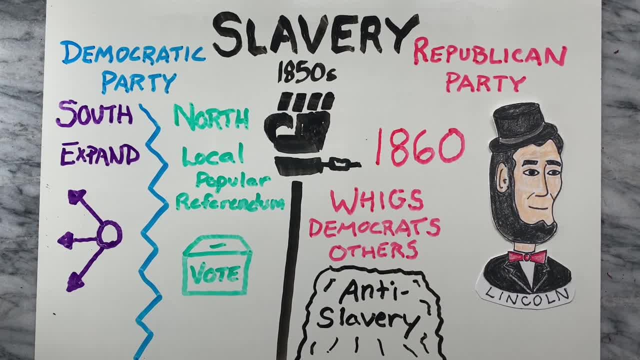 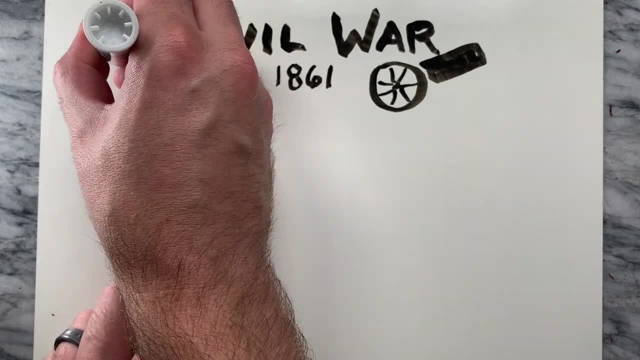 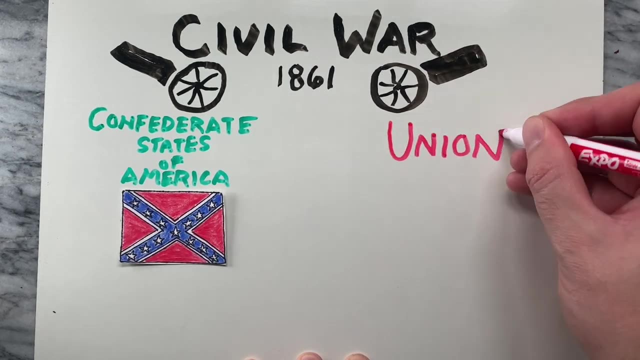 form a party based on an anti-slavery platform. The Civil War broke out in 1861, following President Lincoln's inauguration. In the Civil War, seven southern states formed the Confederate States of America and fought for the detachment from the United States. However, the Union won. the war and the United States was able to win the war. The Union was able to win the war and the Confederacy was formally dissolved. The issue of slavery was at the center of political disagreement during the Civil War, and this caused the Republicans to fight for the abolition of slavery. 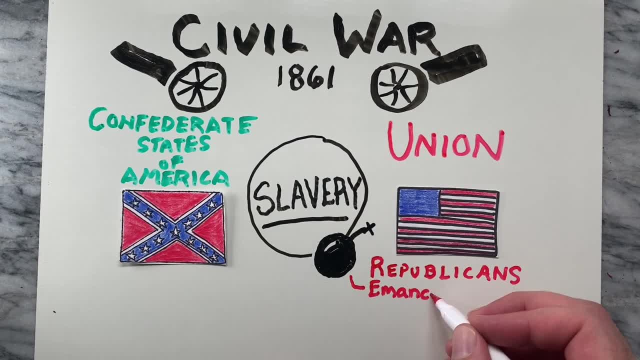 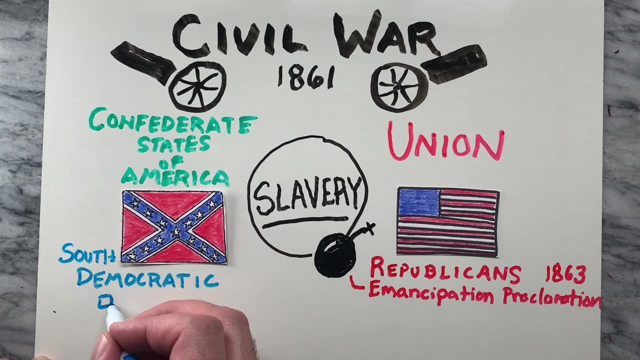 and Lincoln signing the Emancipation Proclamation in 1863.. At this point in history, the South was predominantly Democratic and held conservative, agrarian-oriented, anti-big-business values which were characteristic of the Democratic Party at the time. The majority of the North, on the other hand, were Republicans who fought for civil and voting. rights for African-American people. After the war, the Republican Party became more and more oriented toward economic growth, industry and big business in northern states, and in the beginning of the 20th century it had reached a general status as a party for the more wealthy classes. in society. Many Republicans therefore gained financial success in the prosperous 1920s until the stock market crashed in 1929, initiating the era of the Great Depression. Many blamed Republican President Herbert Hoover for the financial damages brought by the crisis In 1932, the country therefore